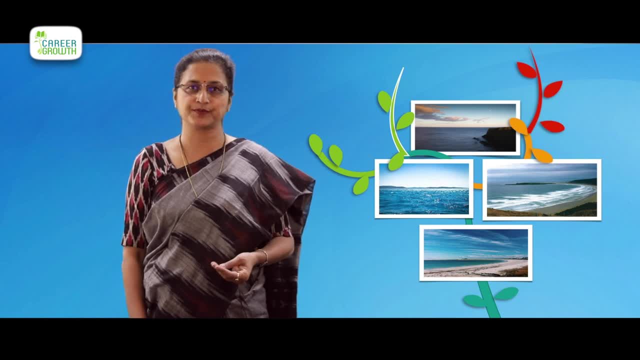 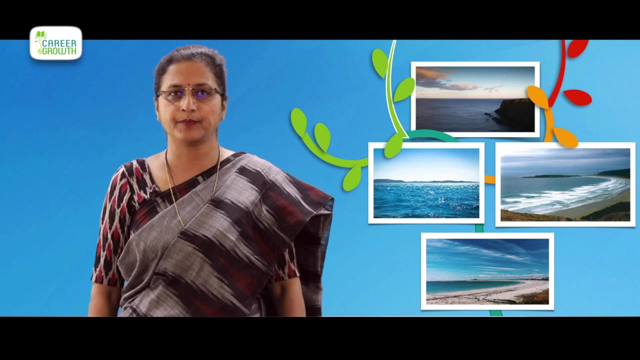 it's a study of ocean and its complex relationships with the planet. it includes the study of weather, ocean currents, sea life and many other topics that are associated with the oceanic or the aquatic life. healthy oceans are crucially important for maintaining a healthy planet. oceanographers are some. 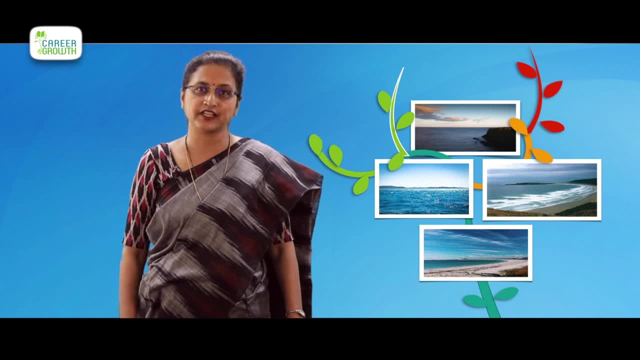 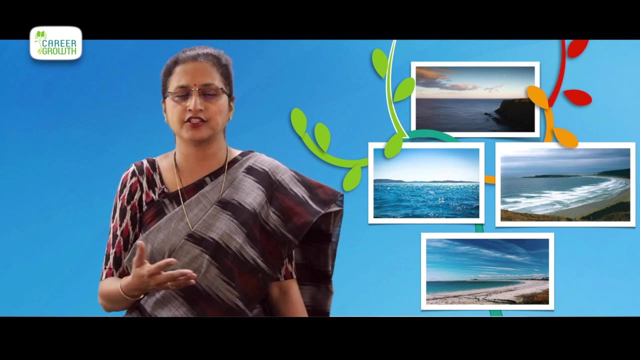 of the important climate researchers in the fight to mitigate the effects of climate change or population and overfishing. remember, oceanographers are also researchers. so what exactly do this oceanographers do? do they stay away from the homeland and are just swimming in the sea, or is it something more? 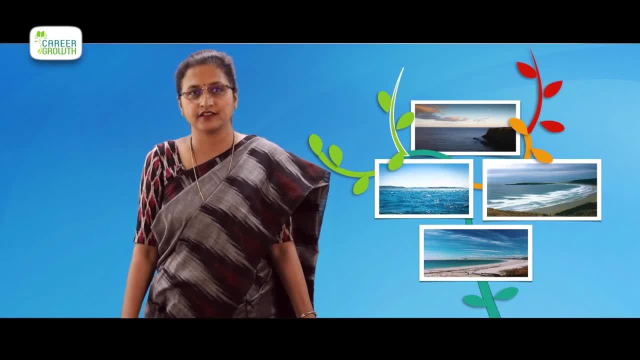 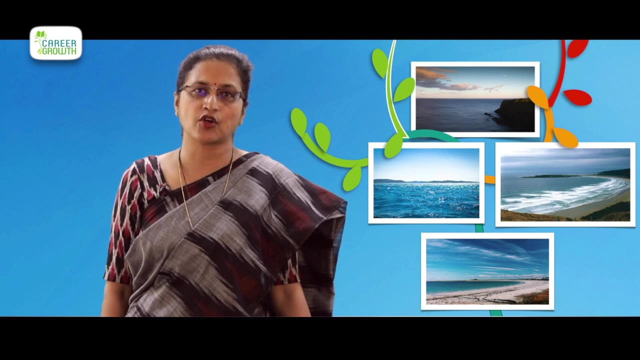 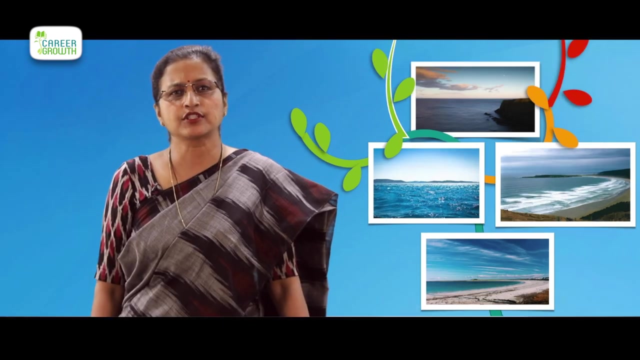 complicated? yes, definitely, the duties are very varied. uh, they plan and carry out field studies in which they visit locations to collect samples and conduct surveys. analyze seawater components, the effects of pollutants and the impacts of chemical processes on marine organisms. conduct laboratory tests on sample collected in the field- I meant the ocean use. 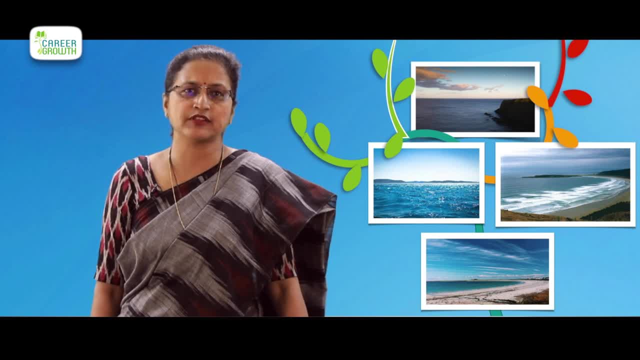 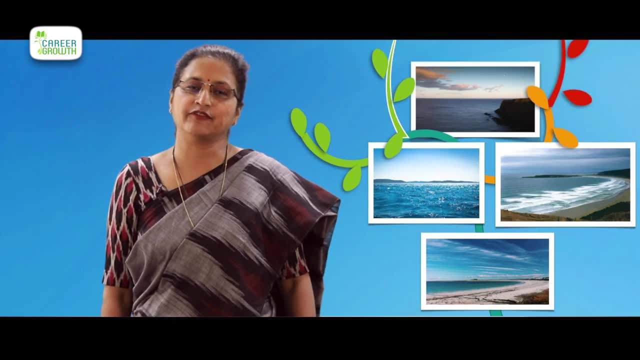 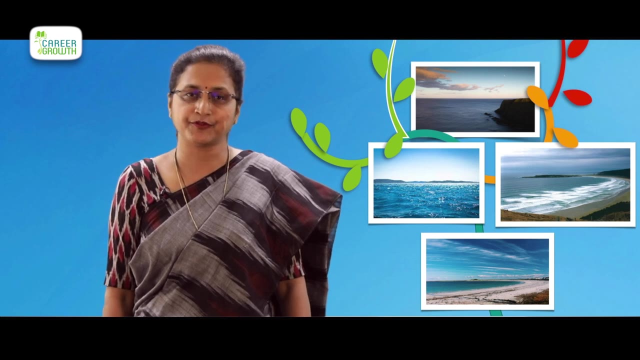 chemistry to understand how ocean currents move seawater around the globe, make geological maps and charts definitely an interesting and one of the most challenging field, as such very few oceanographers into it, but yes, it has been a profession from time immemorial. so how does one get to become? 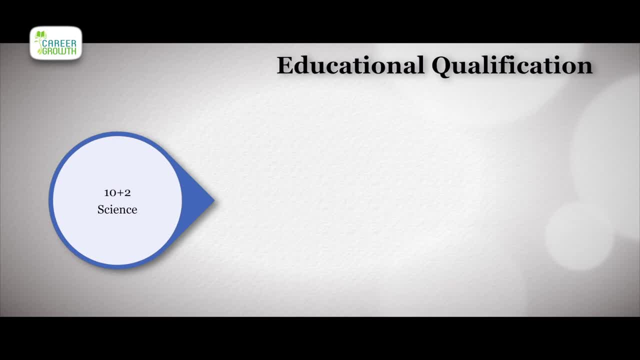 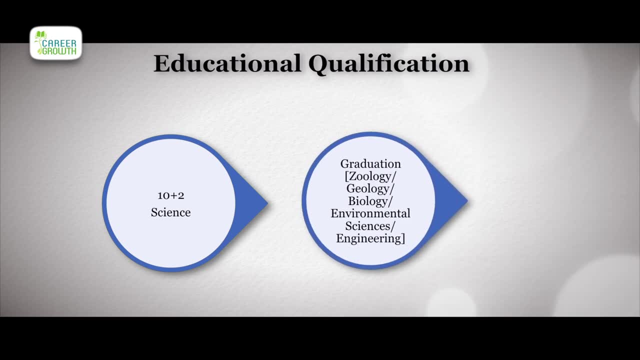 an oceanographer, you need to be a science student right from your plus two level. you could be a graduate in zoology, geology, biology, environmental sciences. you could be an engineer by profession, yes, but the love of oceans have to be learned. you get to learn this interesting degree only at the postgraduate level, at the 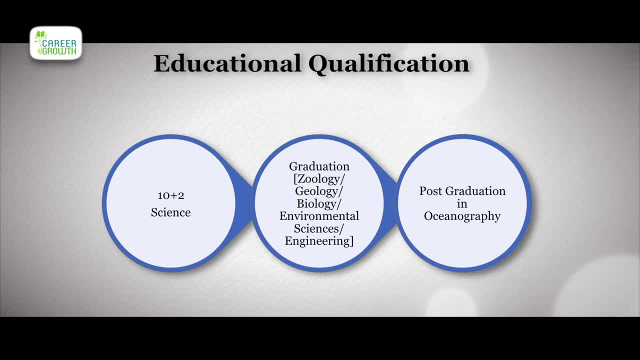 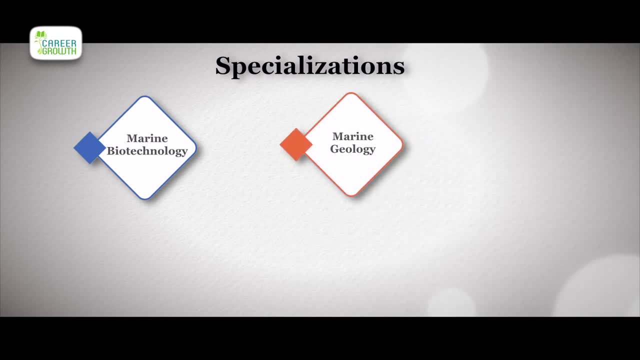 master's, msc or the mtech levels. only you could take up masters and specialize into any of these fields, like marine biotechnology, marine geology, marine geophysics, marine botany, applied geophysics, ocean engineering, marine technology, geotechnology, and so on. and along with the educational qualification,